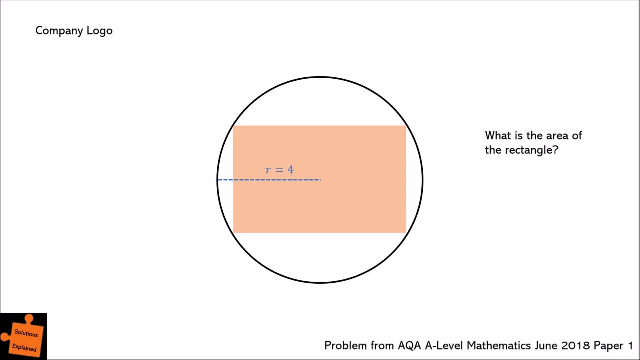 of the rectangle. This problem is from a British A-level mathematics exam designed for 18-year-old students applying to university. If you'd like to have a go at the problem, pause the video and give it a try. Make sure to come back to find out the solution. 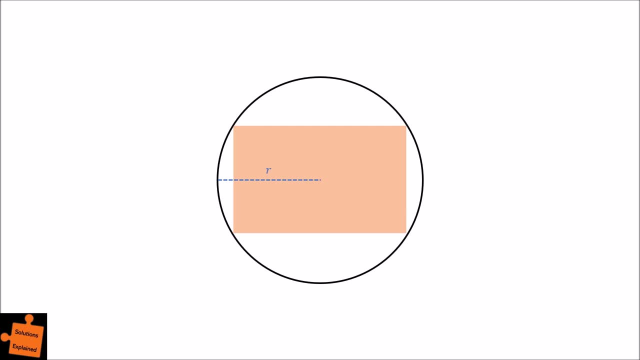 Okay, so let's get started. To begin, we must realise that the radius of the circle is the distance from the centre to any point on the circumference. So we can draw the radius from the centre to the vertex of the rectangle, as shown Now, form a right-angled triangle. 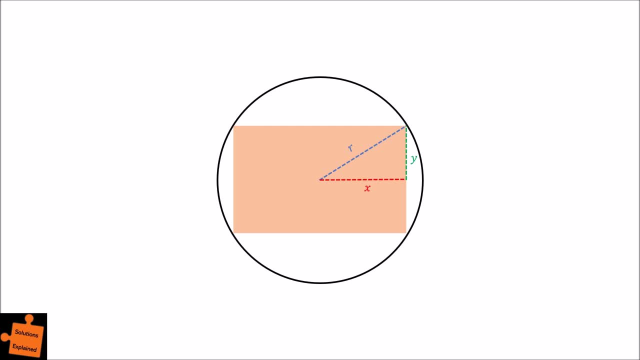 and line it up. We'll label the base and height of this triangle as x and y respectively. By Pythagoras' Theorem we can see that x squared plus y squared is equal to r squared, And this is the general equation of any circle of centre. In this case, r is equal to 4 and thus r squared. 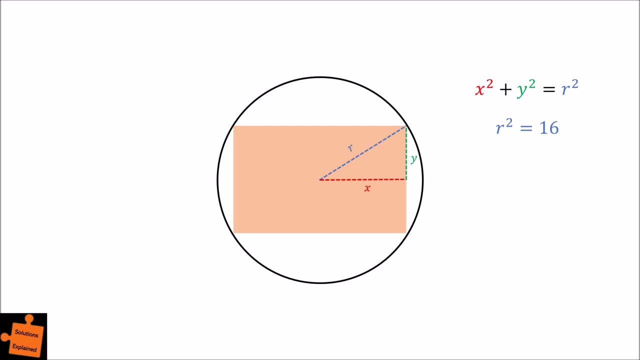 is equal to 16.. And therefore the equation of the circle is: x squared plus y squared is equal to 16.. This equation is satisfied by the following equation: To find the area of the rectangle, it makes sense that we must first find the length and 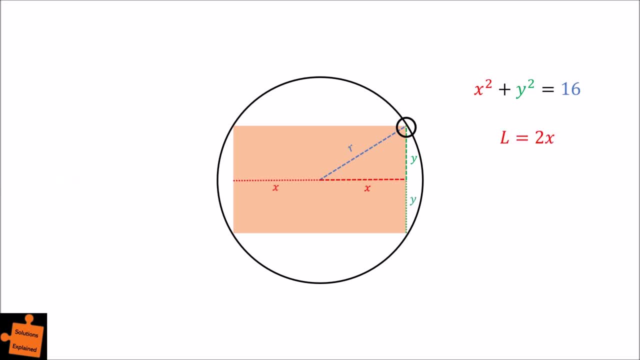 the width. By our notation, the length will be equal to 2x and the width will be equal to 2y, And therefore the area can be written as 2x multiplied by 2y. If we move things out of the way and simplify a little, 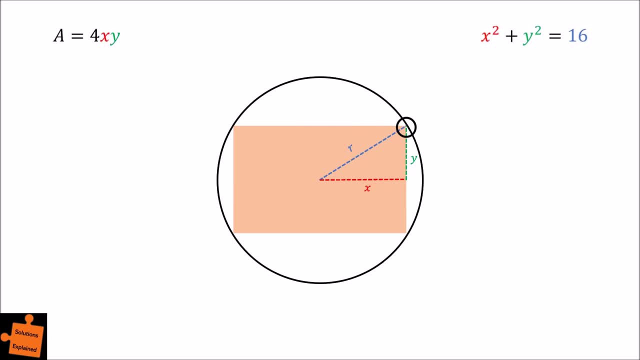 We obtain a circle which is this length and is equal to x squared. If we move this probe, We obtain the area as equal to 4 times x times y. Now we have two separate equations which are both functions of x and y. Let's try and eliminate y to obtain the area purely as a function of x. 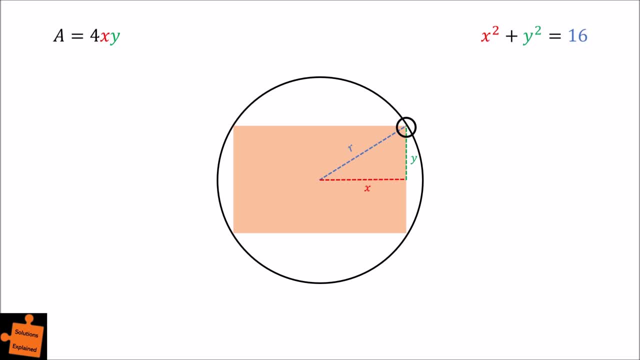 To do this, rearrange the equation of the circle to obtain y as a function of x. Firstly take away the x squared from both sides of the equation and then take the square root to obtain. y is equal to the square root of 16 minus x squared. 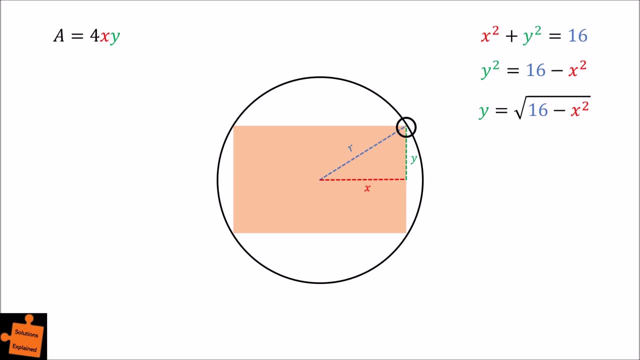 In index notation a square root is the same as a half power, so we can instead write: y is equal to 16 minus x, squared all to the power of a half. This will be useful later on when we need to use calculus. If we tidy this up a little, we can now substitute the equation for y into the area equation. 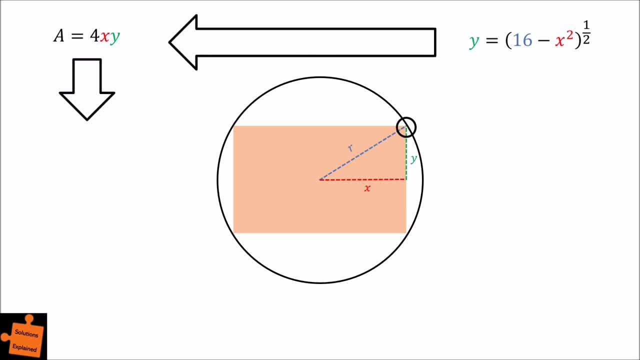 to eliminate y. In doing this we obtain: the area is equal to 4x multiplied by the square root of 16 minus x squared. In other words, we now have the area of the rectangle written purely as a function of x. Let's move the circle out of the way for a moment to focus on this equation for the. 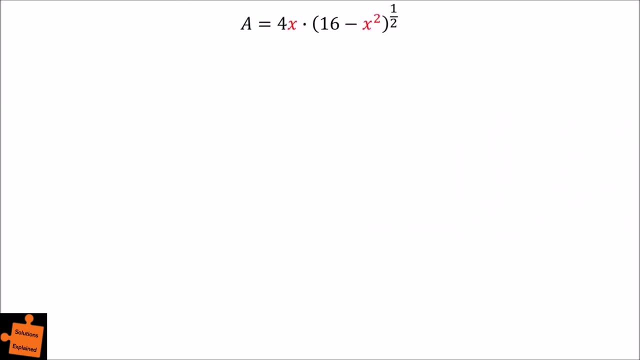 area of our rectangle. We want to find the maximum value of this function. This means we want to find the value of x, which gives the maximum value of a. Let's consider four different values of x and plot these on a graph as we go along. 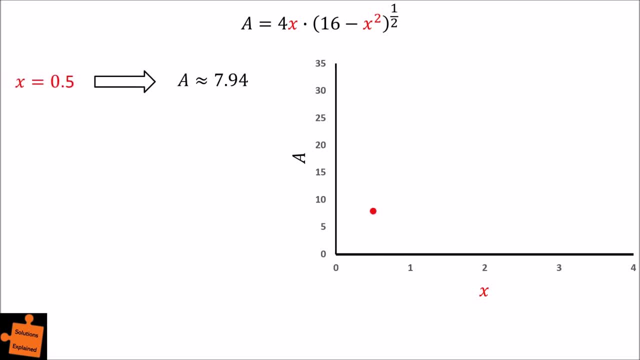 If we plug in x is equal to 0.5, we get a value of 7.9 for the area. If we try x is 1.5, we get a value of 22.5.. If we try x is 2.5,, we get a value of 31.2 for the area. 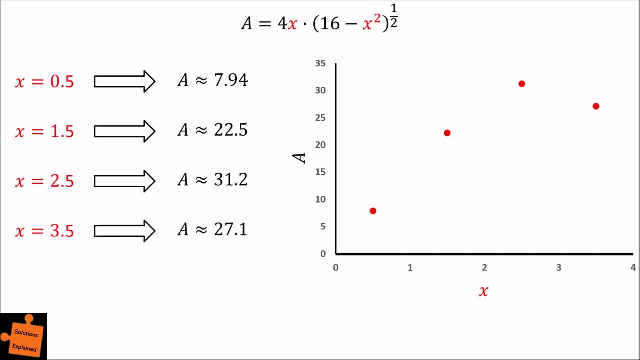 And finally, if we try x is 3.5, we get a value of 27.1 for the area. Let's join these points up using a curve and you can see that there is clearly a maximum point around this section of the graph, somewhere between x is 2.5 and x is 3.5.. 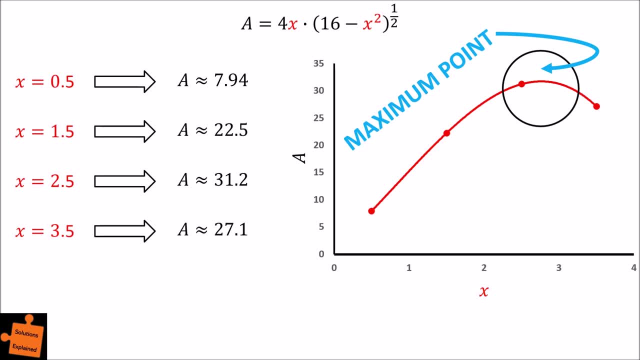 Of course, we could try and read off this x value from the graph, but this is not a very precise way of doing things. Instead, we should use calculus to determine the exact quarter of the x value we want to get from the exact coordinates of the maximum point. 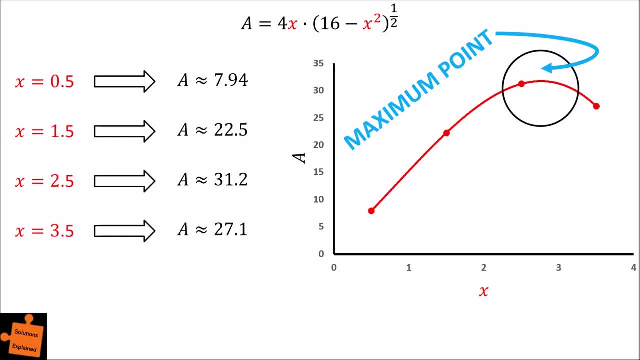 All we need to realise is that, at the maximum point, the gradient of the function is equal to 0. And therefore the next step we need to make is to find an equation for the gradient of our function. To do this, we simply need to differentiate our equation. 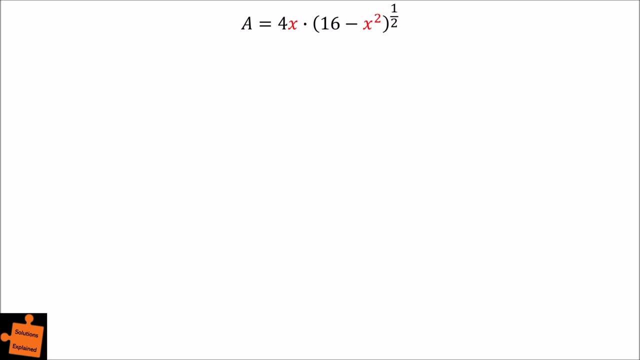 Because our function is actually the product of two separate functions, we need to use the product rule to differentiate our equation. We denote that u is equal to 4x and v is equal to the square root of 16x. Therefore, du by dx will be equal to 4 and dv by dx will be equal to 1 half multiplied. 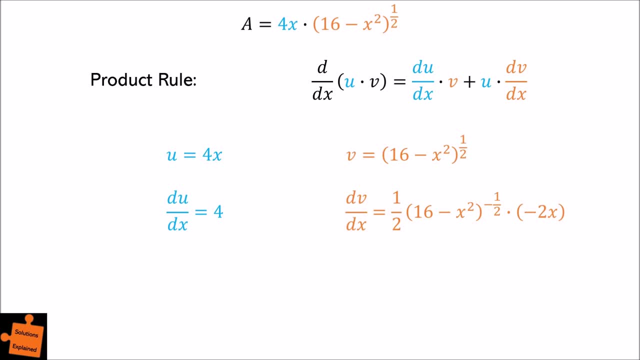 by 16, minus x, squared to the power of minus a half, multiplied by minus 2x. If we simplify this, we obtain: dv by dx is equal to minus x multiplied by 16, minus x, squared to the power of minus a half. We can now substitute all of this into the formula for the product rule to obtain an. 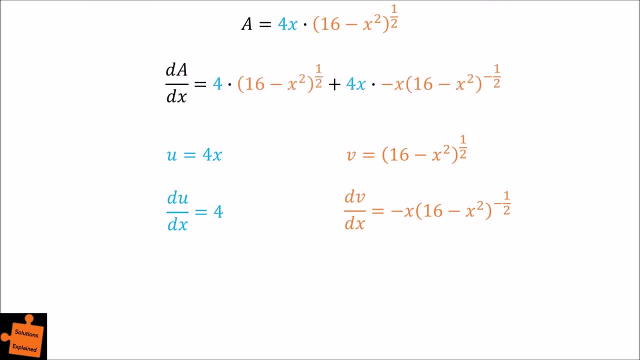 equation for the gradient dA by dx. If we run through the maths and simplify this equation, we obtain that dA by dx is equal to 64 minus 8x, squared, all over the square root of 16 minus x squared. Recall that at the maximum point the gradient is equal to 0 and thus dA by dx is equal to. 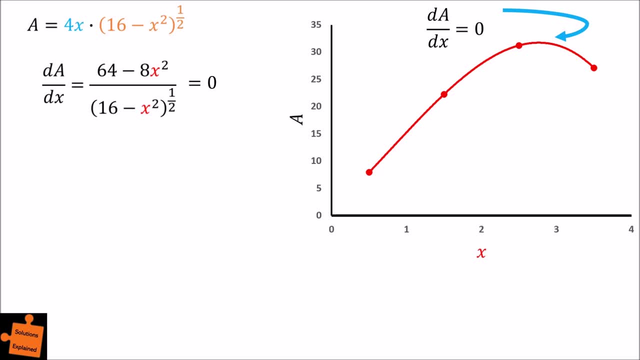 0.. Therefore we can set the gradient function as equal to 0 and then rearrange this to find the value of x which results in the maximum error. Firstly, multiply up by the denominator to obtain 64 minus 8x squared is equal to 0.. 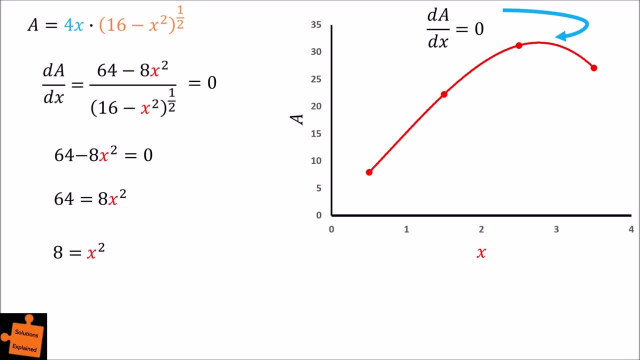 Take the 8x squared to the other side and then divide by 8 to obtain that 8 is equal to x squared. Finally, take the square root to find that x is actually equal to 2 root 2, which is approximately 2.83 and is shown on our graph here on the right. 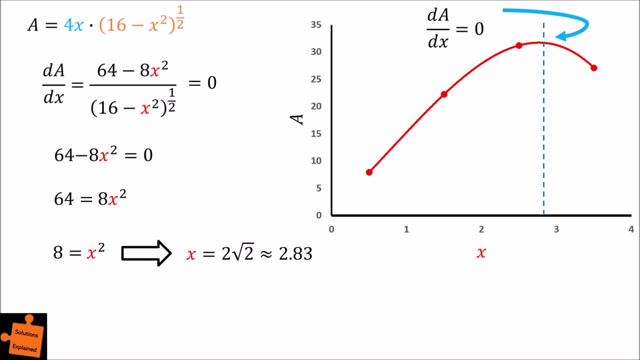 This is the value of x which results in the maximum error. If we now take a look back at the circle and rectangle logo, we can conclude our problem. We can now take a look back at the circle and rectangle logo. we can conclude our problem. 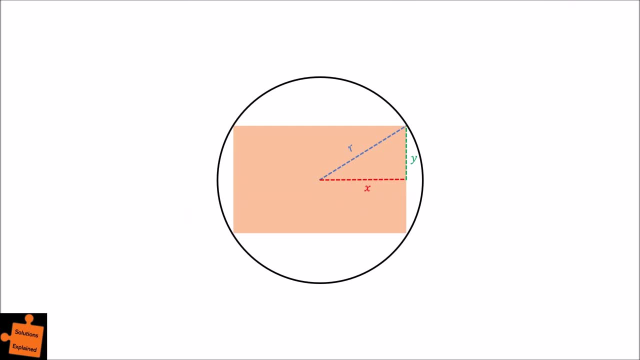 We can now take a look back at the circle and rectangle logo. we can conclude our problem. We can now take a look back at the circle and rectangle logo. we can conclude our problem. So we know that x is equal to 2 root 2.. 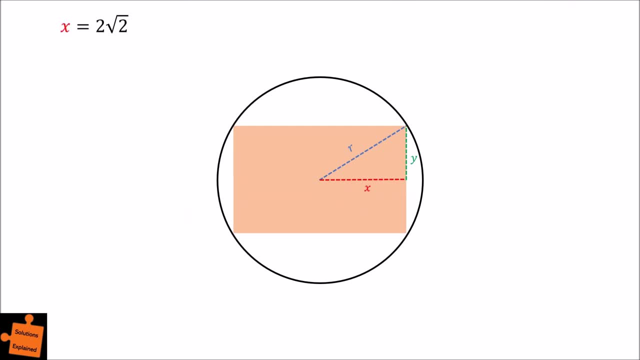 Recall that from the equation of the circle. we can write y as equal to the square root of 16 minus x squared. Substituting x is equal to 2 root 2 into this equation and we obtain a surprising result: y is also equal to 2 root 2, and so the rectangle in our logo is actually a square. 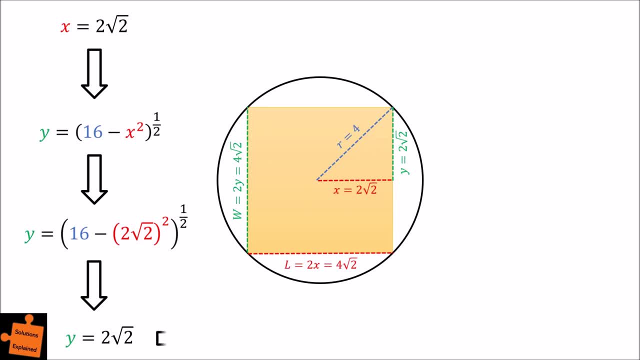 This square will have side length 4 root 2 and thus the area of our square will be 4 root 2 multiplied by 4 root 2.. This gives an area of 32.. This is the final answer to our question. 32 is the maximum area of a rectangle inside a circle of radius 4, and the rectangle will